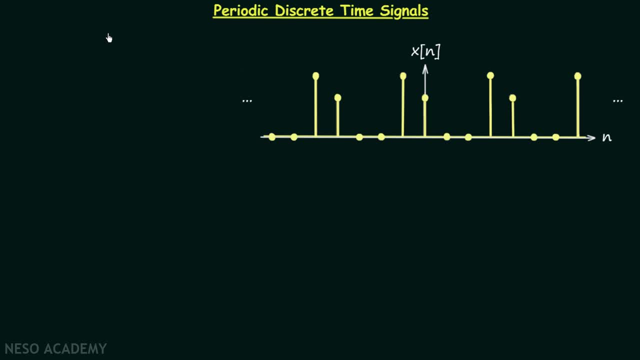 exponential discrete time signal and sinusoidal discrete time signal to be periodic. So let's begin with the first very important question, ie what are periodic discrete time signals? A discrete time signal is said to be periodic if the signal remains the same after performing the left shifting operation and the right shifting operation by k times. 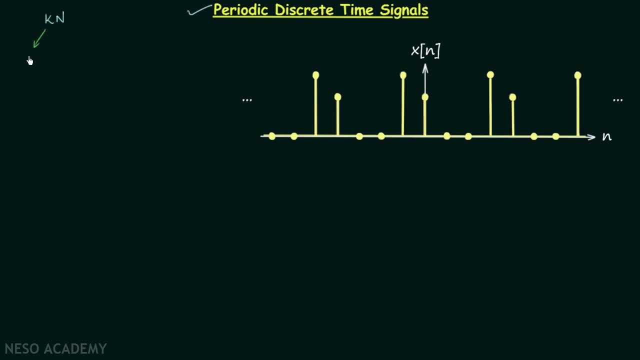 n, k is an integer and n is known as the fundamental time period of the discrete time signal and, like k, n is also an integer. This is one important point: that the fundamental time period, n, is an integer. So whenever we perform the time shifting operation, whether the left shifting, 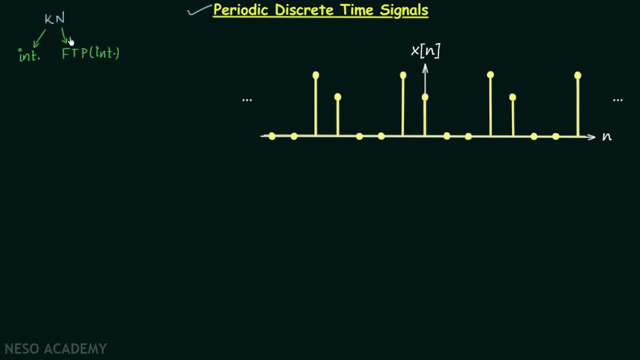 or the right, shifting on a discrete time signal by k, n, and we have the same signal. then we will see that the signal we are having is periodic in nature. To understand this point, let's take one signal- xn- This is the discrete time signal- and let's say the signal is having the fundamental time period equal. 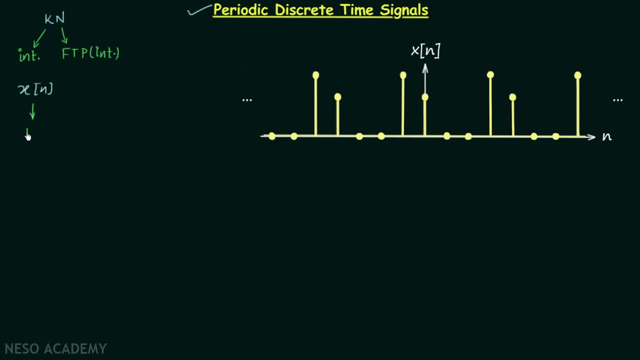 to n. This is having the fundamental time period equal to n. and now, if we perform the left shifting operation by k times n, we will have a new signal xn plus k times n. and if we perform the right shifting operation by k times n, we will have a new signal xn minus kn. and if these two signals are same as the, 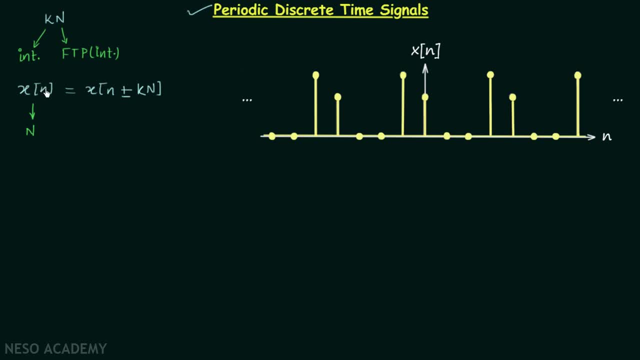 initial signal xn. we will say that signal xn is a periodic signal. So this is the condition for a signal to be periodic signal and using this condition we can calculate the fundamental time period n. Now we will understand why we are having the same signal after performing the right shifting. 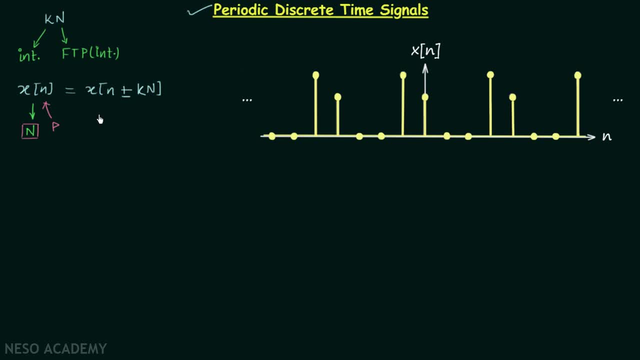 and the left, shifting by k times n. And for this I have to do this. I have taken one example waveform. this is the waveform of signal xn and you can see that in this waveform one particular structure is repeated from minus infinity to plus infinity, and we know the fundamental time period: n is the extension of the smallest repeated. 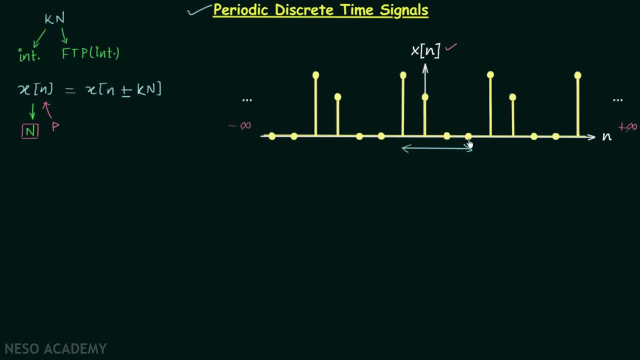 structure, Which, in this case, is this structure And therefore Our signal. xn is equal to 2 minus minus 1, and then plus 1.. Plus 1 is for n equal to 0. This will give us n equal to 4.. 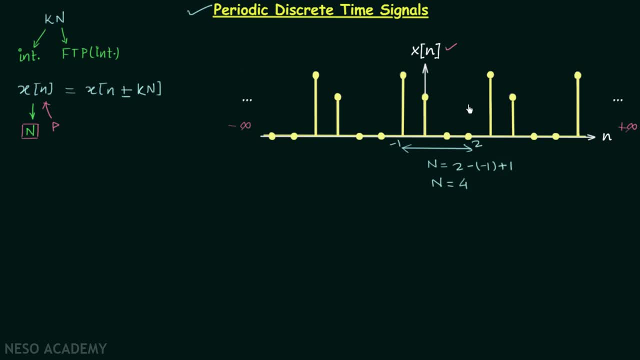 Therefore, when you perform the left shifting or the right shifting of this signal by the integer multiple of 4, you will get the same signal. This implies, if you perform the shifting by k times 4. You will have the same signal. and to understand this, let's say k is equal to 1. this will give you 4, so perform the left shifting. 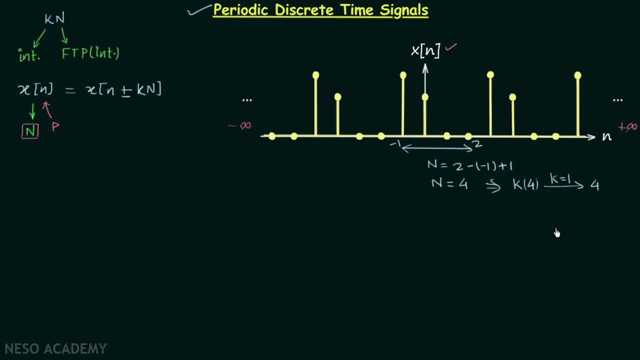 or the right shifting by 4 and you will find you have the same signal. you know how to perform the shifting operation and therefore you can do this by yourself. and after performing the shifting you will have the same signal. and this is happening because the same type of a structure is repeated. 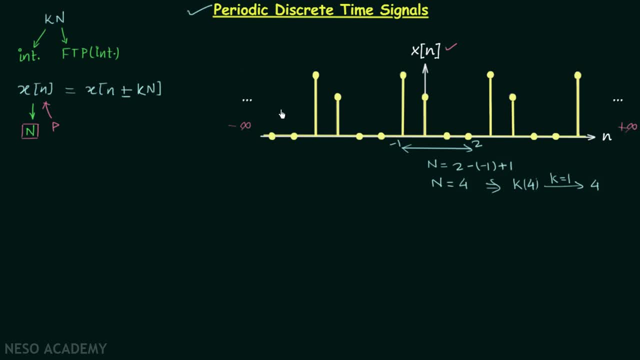 from minus infinity to plus infinity. if this repetition is not from minus infinity to plus infinity, you will not have the same signal. therefore, for all the periodic signals, a same type of a structure, or you can say a particular structure, is repeated from minus infinity to plus infinity. this particular condition is very important. so 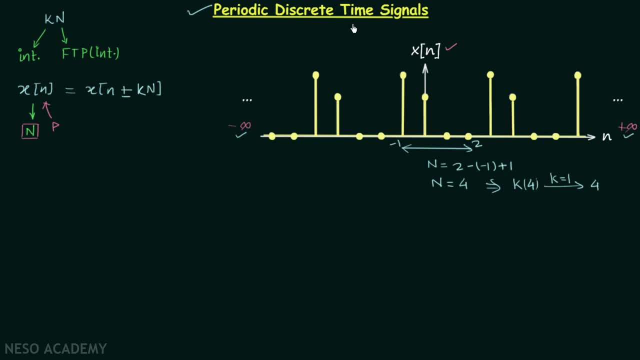 i hope you now understand what are periodic discrete time signals and the condition for a discrete time signal to be periodic. now we will move on to the next part of this lecture and in this part we will talk about the composite discrete time signals. let's say signal xn is a. 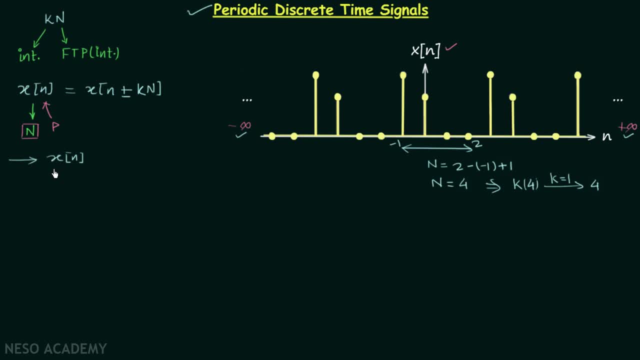 composite discrete time signal, and by composite signals we mean it is obtained after combining two or more signals, and signal xn is, let's say, equal to x1n plus x2n. x1n is a periodic signal and this signal is having the fundamental time period equal to n1. x2n is also a periodic signal, having the fundamental. 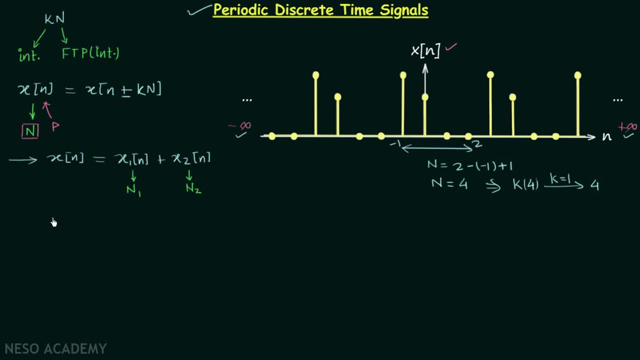 time period equal to n2. now, if you try to remember, while discussing the periodic continuous time signals, i told you that if there is a composite continuous time signal xt, which is equal to continuous time signal x1t plus continuous time signal x2t, and signal x1t is a periodic continuous time signal with the fundamental period equal to t1 signal x2t. 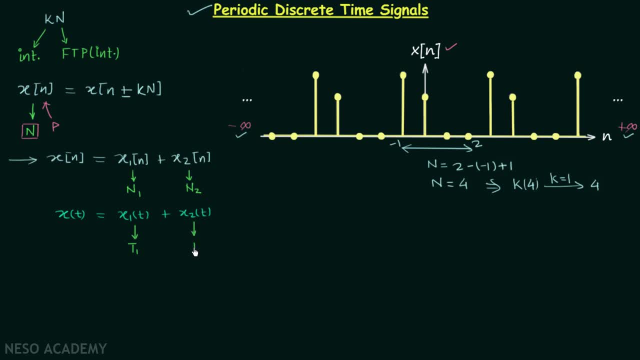 is also a periodic, continuous time signal with the fundamental period equal to t2, then this signal, composite signal xt, will be periodic, will be periodic only when, only when, the ratio t1 by t2 is a rational number and this signal, this signal, will be a periodic. 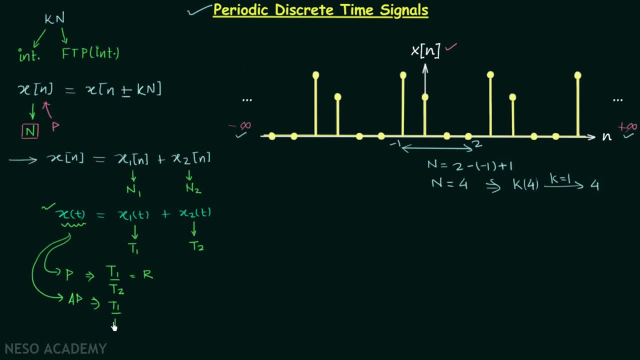 what is highly valuable. if the ratio t1 by t2 is an irrational number. the same thing is applicable in case of composite discrete time: signal xn: the ratio and one by n 2. the ratio and one by n 2. if rational, then this implies signal xn. 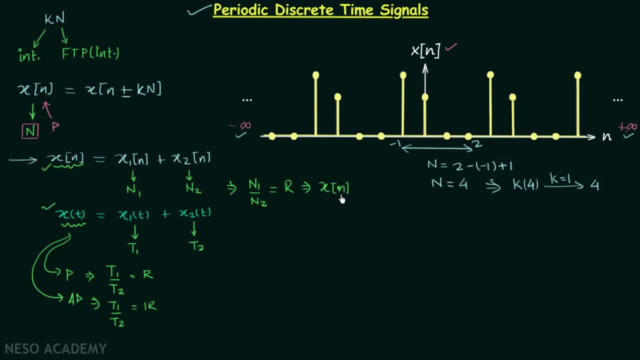 miners also. map xn is periodic, and if the ratio n1 by n2 is an irrational number, then this signal xn is aperiodic. and when signal xn is periodic, then we go on calculating the fundamental time period, n. and if it is aperiodic, then this: 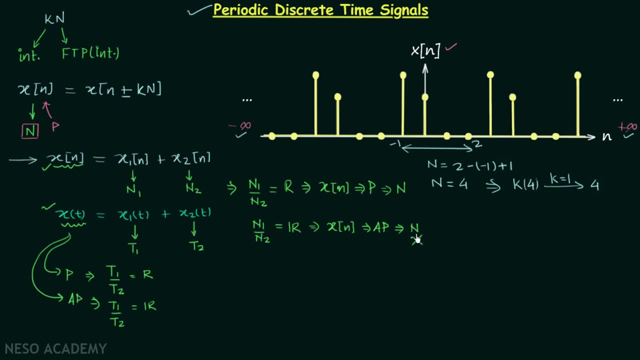 implies there will be no fundamental time period, n. now there is one catch. we know: n1 is an integer. I have already told you, n is an integer, the fundamental time period is an integer, so n1 is an integer. n2 is also an integer, so the 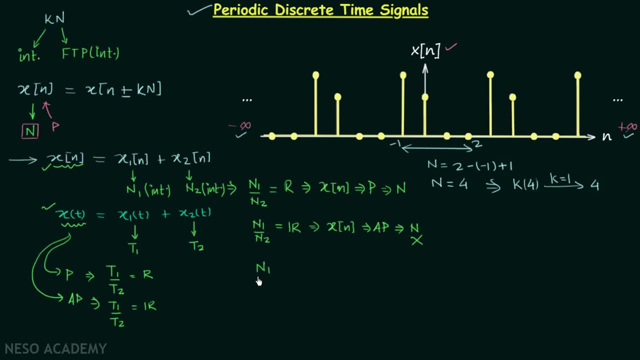 ratio n1 by n2 we are talking about is simply equal to an integer by an integer, and we know integer by an integer is always going to be rational. so the ratio is always going to be rational. and whenever the ratio is rational, signal xn is periodic. so this implies our composite signal, which is a. 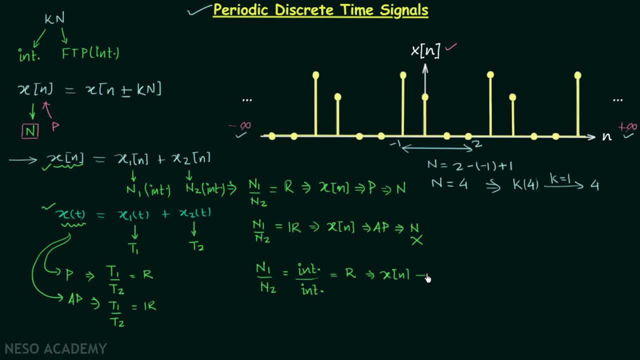 composite discrete time signal is always going to be periodic in nature. so whenever you are dealing with composite discrete time signals, there is no need to check whether the ratio is giving you the rational value or the irrational value. simply move on to the calculation of the fundamental time. 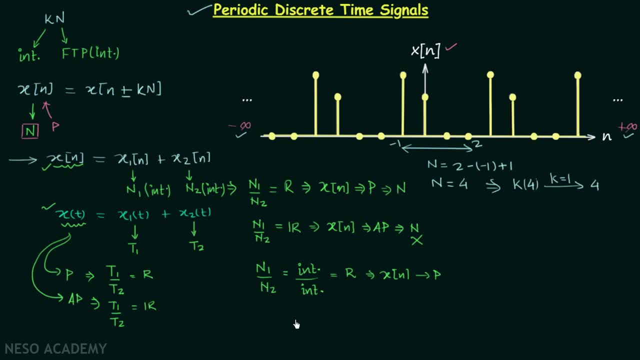 period of xn, which is n, and we know how to calculate n. n, which is the fundamental time period of the composite signal, is equal to LCM of n1 and n2. so once you solve this, you will have the fundamental time period n. so this is all for the second part, and now we 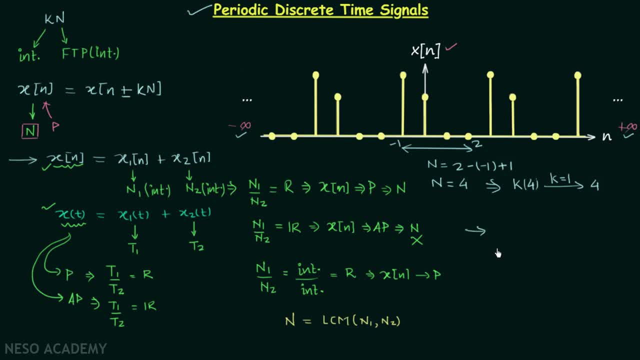 will move on to the third part of this lecture and in this part we will try to understand what is the condition which must be satisfied for all the complex exponential and sinusoidal discrete time signals to be periodic whenever you have a continuous time- sinusoidal signal or continuous- 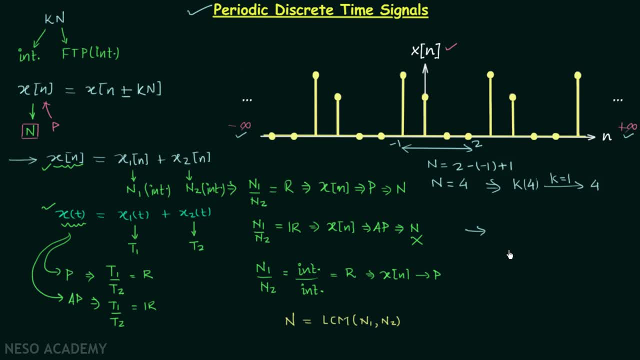 time, complex exponential signal, they are always periodic. but discrete time, complex exponential and discrete time sinusoidal signals are not always periodic. there is one condition, and now we are going to derive that condition, and for this we will take one signal action which is equally war тутo, which is nothing unlike that one. then we can have that condition in this picture. 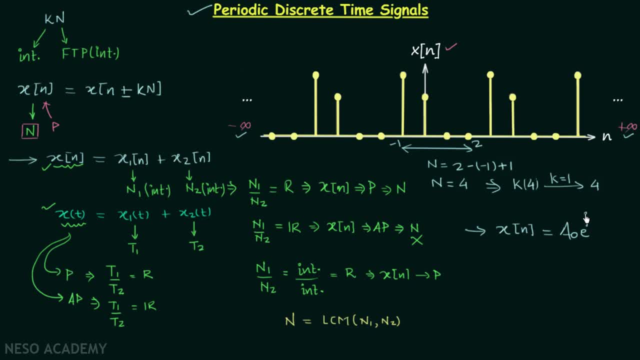 and you will tell me more about the second part of this. now we will go to the third part and說- and this we will explain twoQuickly and four to the Curt зав Broken- Why in one the two parts equal to a0, e, power, j, omega0n. and we know the condition for this signal to be periodic. 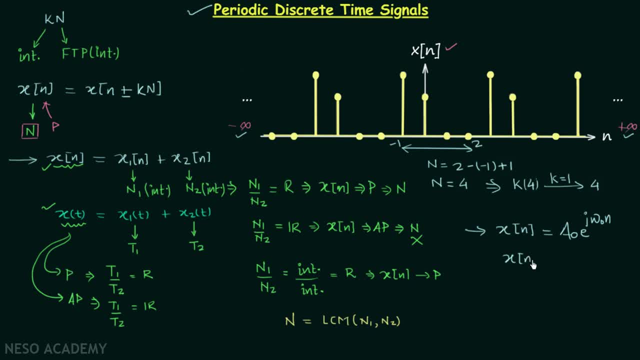 This is the condition, So xn should be equal to xn plus kn. You can consider the case of right shifting as well, but I have considered the case of left shifting and we know xn is equal to this. So on the left hand side we will have a0, e, power, j, omega0n, and on the right hand side 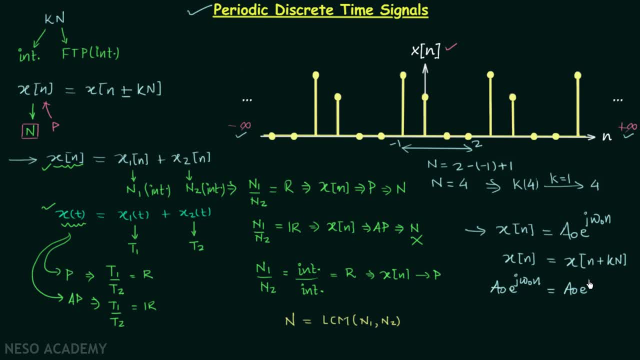 we will have a0, e, power, j, omega0.. In place of n, we will write n plus kn. Let's say k is equal to 1, to simplify the things. So we will have n plus n. and now, in the next step, I will separate the exponentials. 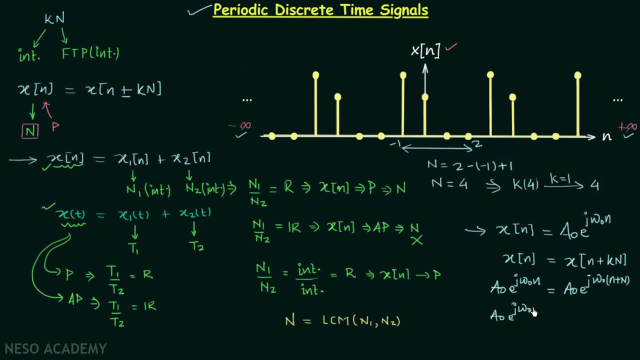 So we have a0 e power j omega0n on the left hand side, and on the right hand side we will have a0 e power j omega0n multiplied to e power j omega0. capital N e power j omega0n multiplied to a0 will be cancelled out, so we are left with 1 equal. 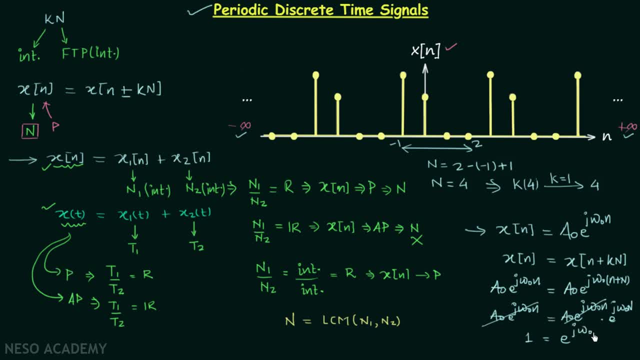 to e power, j omega0n, e power, j- omega0n. And we can write 1 equal to e power, j 2pi k. Now, on comparison, you can see that omega0n- omega0n is equal to 2pi k. 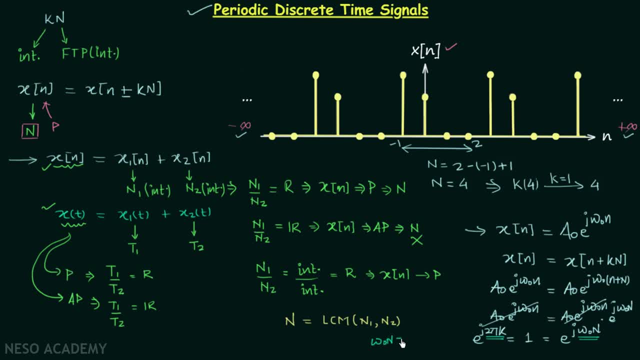 So here I will write down: omega0n is equal to 2pi k and we can say that 2pi, 2pi divided by omega0.. Here, an ascendant order symbol, Lakshmi, is equal to n by k, and n by k will give you. 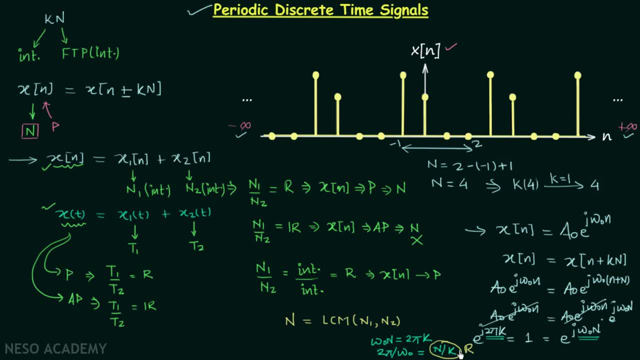 r for help, because n is an integer, k is an integer. integer by integer will give the ration number. So 2pi divided by omega0 will give you the rational number. if complex exponential signal you are having or the sinusoidal signal you'are having is periodical, 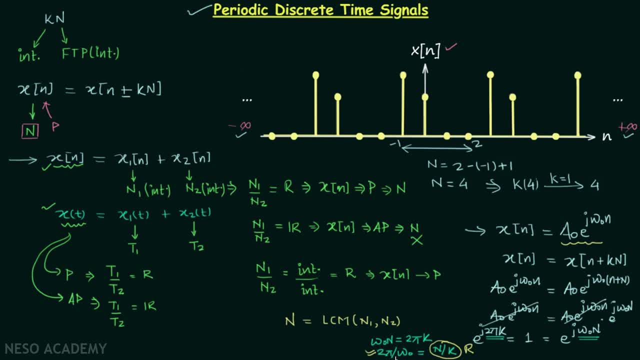 Now, in this case, whether we will be safe at the, It will not make difference to nowhere because it will not assume part and part one will be fine. So this is the condition for discrete, complex exponential and discrete sinusoidal signals to be periodic. 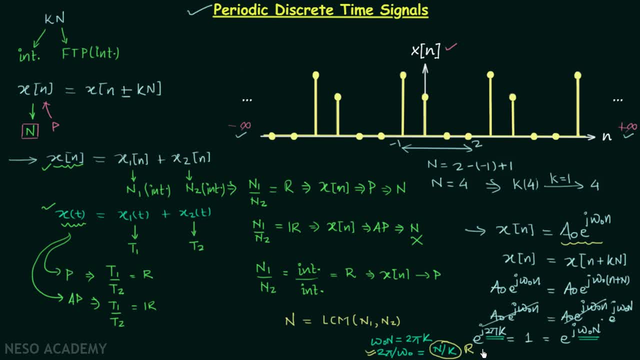 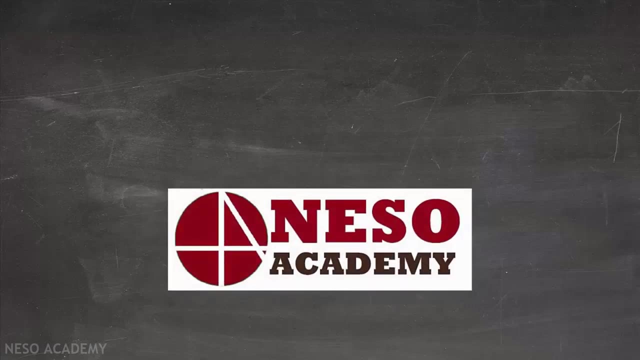 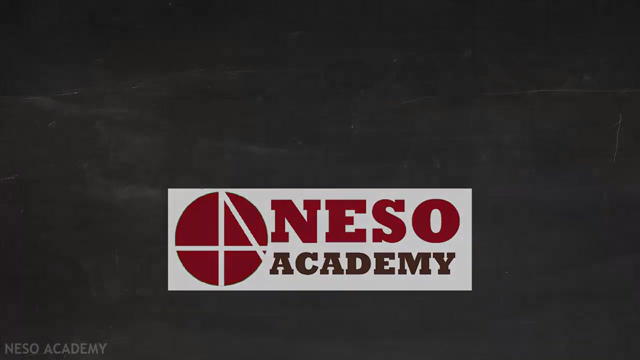 Ratio of 2, pi and omega naught should be rational. So this is all for this lecture. In the next lecture we will solve few questions based on the concepts we have developed in this lecture. Thank you for watching. 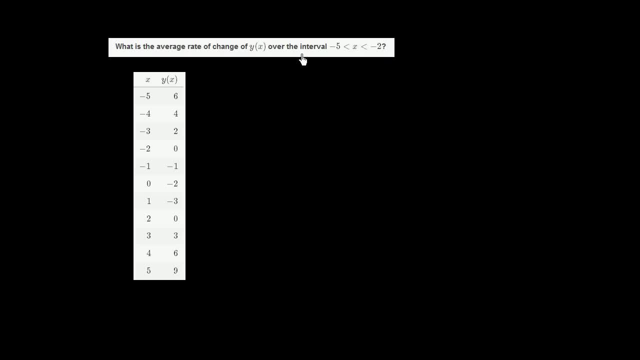 What is the average rate of change of y of x over the interval? negative 5 is less than x is less than negative 2?. So this is x is equal to negative 5.. When x is equal to negative 5, y of x is equal to 6.. 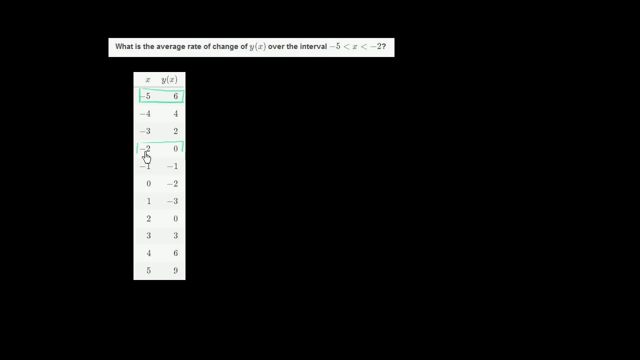 And when x is equal to negative 2, y of x is equal to 0.. So to figure out the average rate of change, so the average rate of change of y of x, with respect- and we can assume it's with respect- to x. 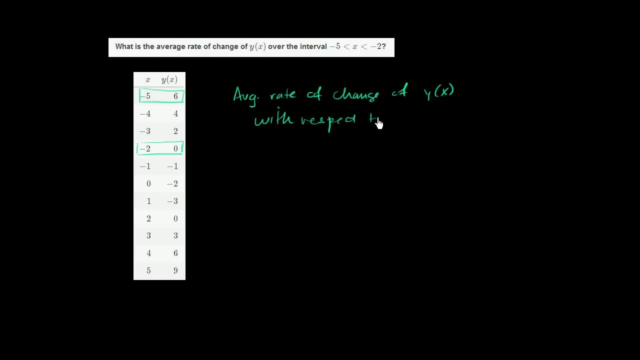 with respect to x. let me make that a little bit neater. with respect to x, this is going to be the change in y of x over that interval, over the change of x of that interval, And the shorthand for change is this triangle: